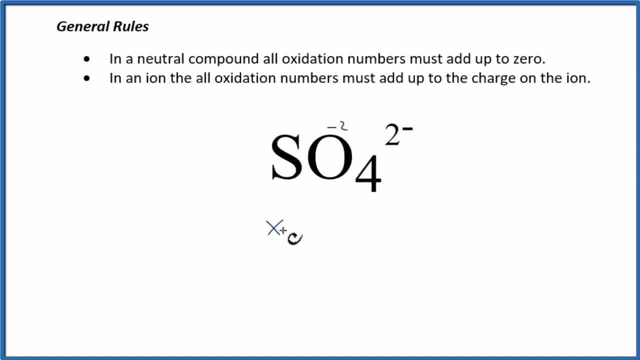 We know oxygen has a minus 2 oxidation number. so we say sulfur, that's X plus minus 2 times 4, we have 4 oxygen atoms equals the charge on the ion. So we solve for X and we find that X equals plus 6,. 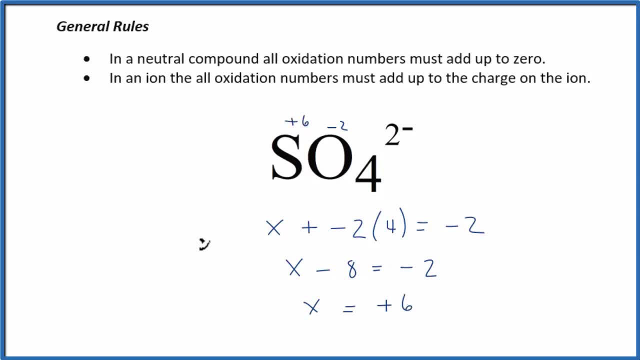 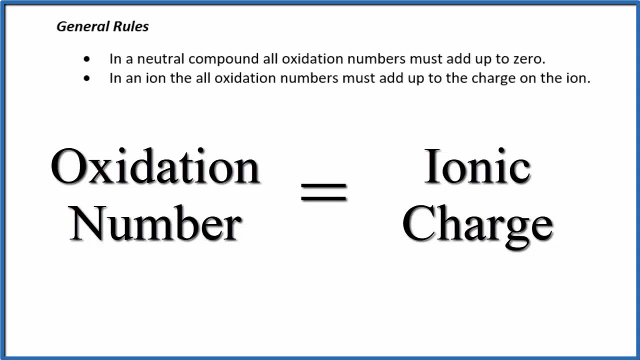 and that's the oxidation number on the sulfur in SO4: 2 minus. Speaking of oxidation numbers and ionic charge, the big thing to remember is that, while they do overlap, some oxidation number and ionic charge are not the same thing. For example, the ionic charge for nitrogen is always going to be 3 minus. 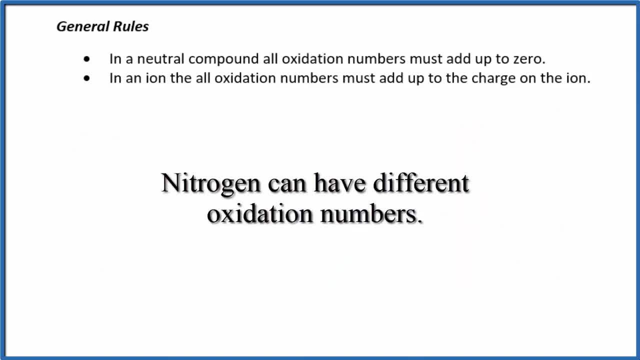 When we look at the oxidation number for nitrogen, it changes. It can be different things. For example, in N2O it's plus 4, but in NO it's plus 2.. The key thing to remember: oxidation numbers and ionic charges are not the same thing. 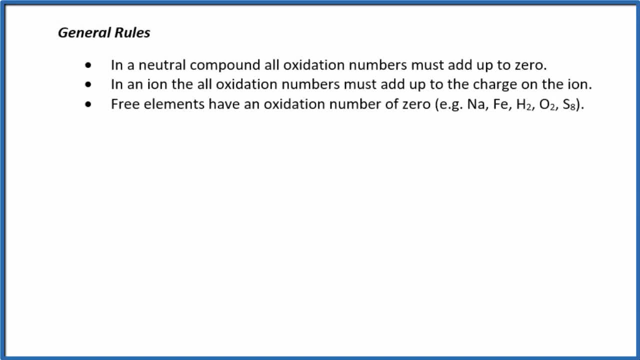 The next rule, it's easy: The oxidation number for free elements, also called monatomic substances, where there's only one type of atom in the substance, those are zero. So pause and find the oxidation number for these substances. Remember, for ions like Ca2 plus or F minus, the oxidation number is equal to the charge. 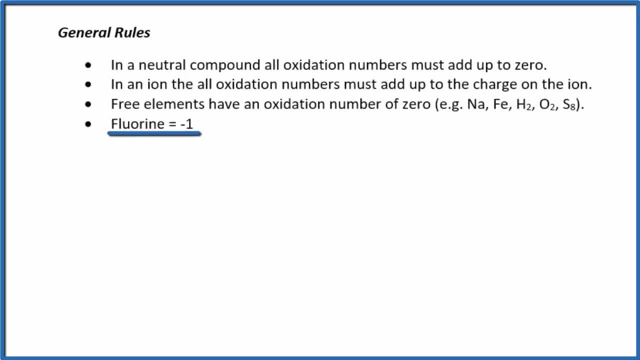 Another straightforward rule is that fluorine F is always minus 1.. Pause and give these a try. So in the first one- this is a little strange, Here we have oxygen is plus 2, but that's because fluorine is always going to be minus 1.. 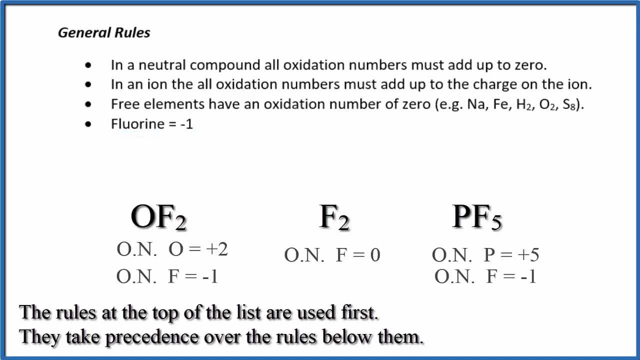 Two fluorines 2 times minus 1, that's minus 2.. The oxygen has to be plus 2.. And I hope I didn't catch you with the F2 here. It's a neutral compound and all the atoms are the same, so its oxidation number is zero. 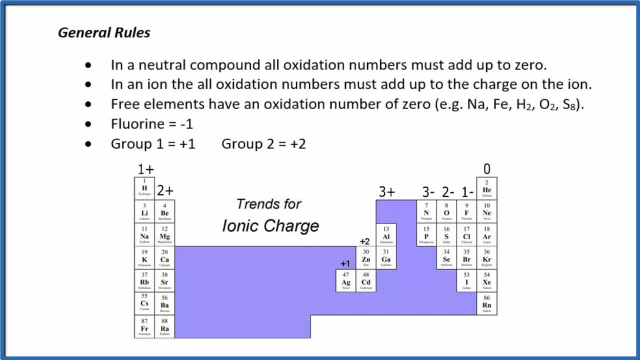 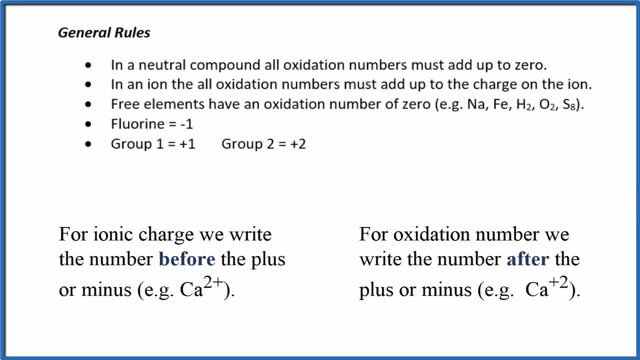 In this next rule, oxidation number and ionic charge do overlap On the periodic table. elements in group 1 have a 1 plus charge. Their oxidation number is plus 1.. Group 2 has an oxidation number of plus 2, and aluminum in group 13,, sometimes called 3A, is plus 3.. 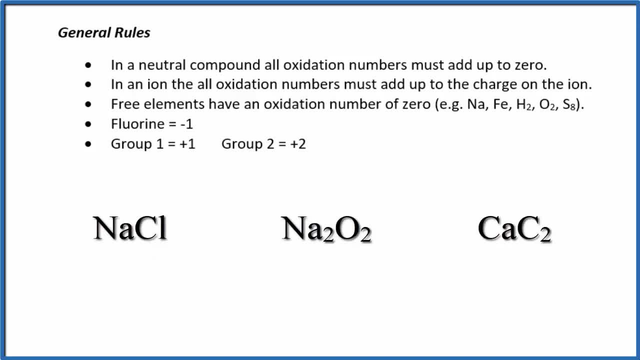 So pause and try these. Note that for Na2O2, sodium peroxide, oxygen doesn't have a minus 2 charge. Here it's minus 1.. Peroxides: they're an exception for the rule that oxygen has a minus 2 oxidation number. 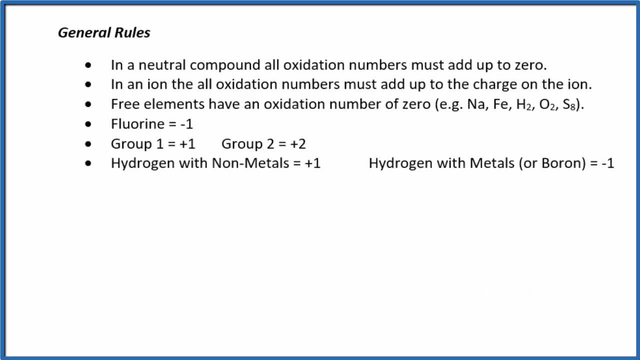 I mean, how many more rules are there? Just a few. An important one is that hydrogen has a plus 1 oxidation number when it's bonded to nonmetals. When it's bonded to metals, it's minus 1.. Here's the periodic table, divided into metals and nonmetals. 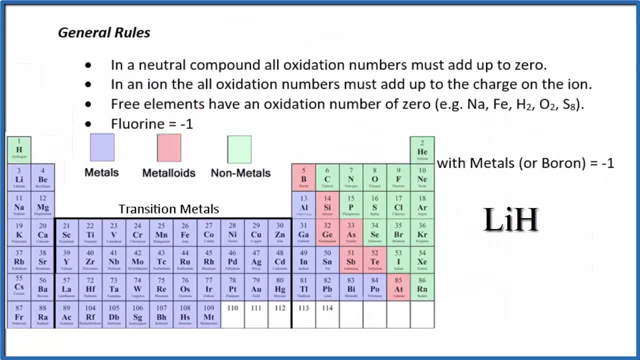 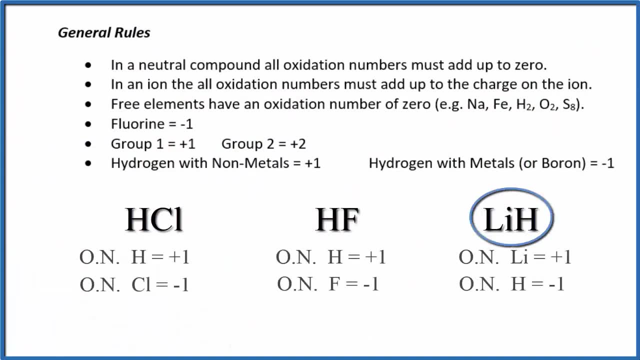 So pause and find the oxidation numbers for the elements in these compounds. Note that in LiH the hydrogen is negative and it's written after the metal, after the lithium. Okay, two more rules. This one's important Oxygen is usually minus 2, with two big exceptions. 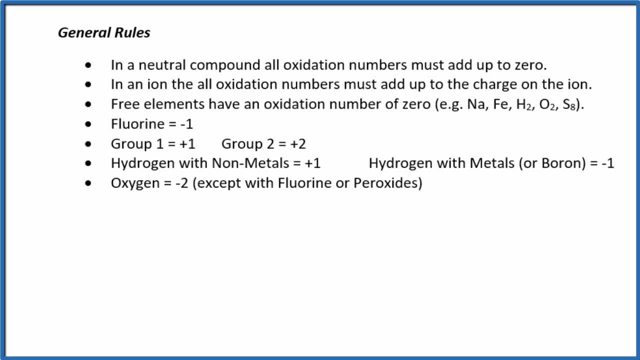 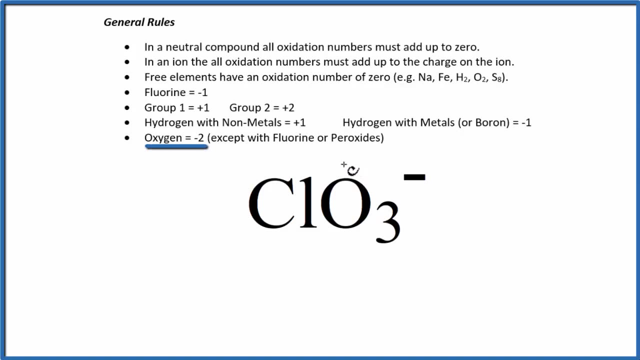 Do you remember them When bonded to fluorine and in peroxide? So pause and find the oxidation numbers for each element in these compounds. Let's give ClO3- a try. We know that oxygen has an oxidation number of minus 2.. 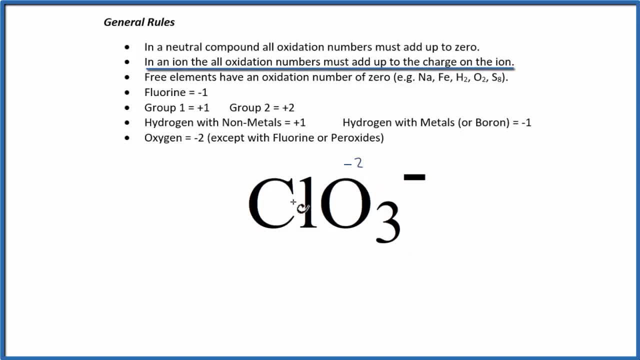 We also know that we have an ion here. So all the oxidation numbers are going to add up to the charge on the ion. So let's figure out the oxidation number for chlorine. We could say chlorine, call that x minus 2.. 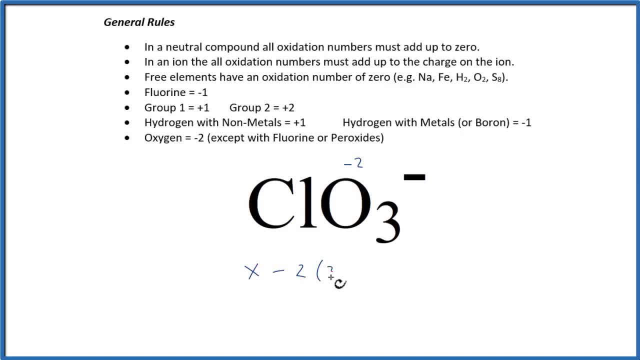 We could say chlorine, call that x minus 2.. We could say chlorine, call that x minus 2.. For the oxygen there are three: oxygen atoms equals the charge on the ion minus 1.. x minus 6 equals minus 1.. 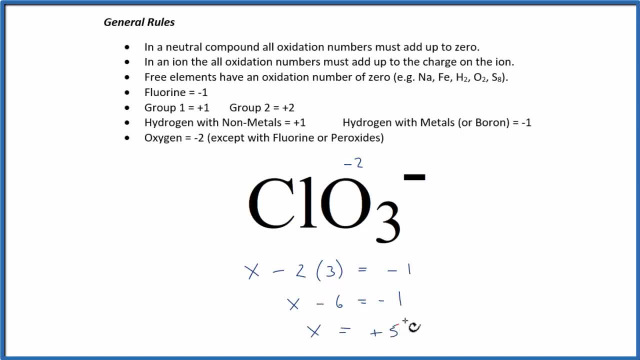 x, that equals plus 5. And that's the oxidation number on the chlorine. So we found the one that we knew, the oxygen, which is minus 2.. We know that it all has to add up to a negative 1 because of the charge here. 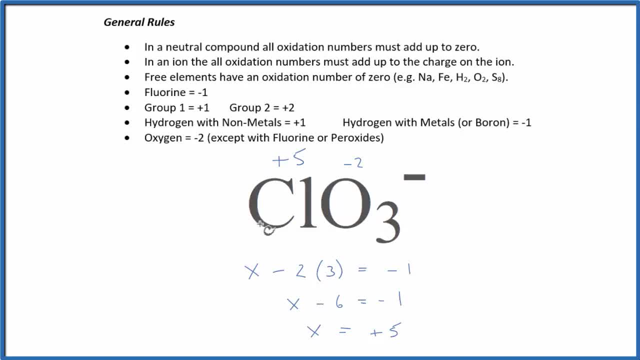 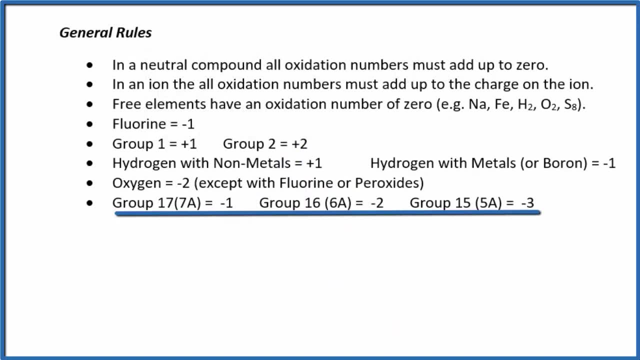 And we use that information to find the oxidation number on the chlorine. The last rule: If none of the rules above apply, you can use these rules in this order. So pause one last time and give these a try. So we've done a bunch of practice in this video.